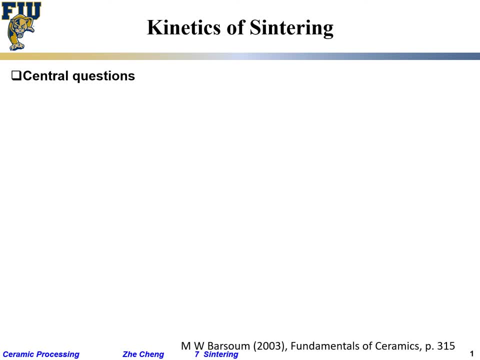 Okay, so after we talked briefly about the magnetism, let's talk about the kinetics, And people study kinetics, which is essentially: how fast does things go? The central question would be: how do ceramic bodies change in their density with respect to time, or how does ceramic body 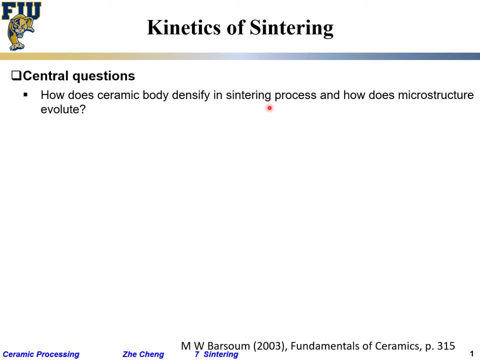 densify in this centering process? with respect to time, right, How fast do it happen? And, at the same time, how does the microstructure- green size, green shape, pore size, pore shape- change or evolute? okay, And the related question is: 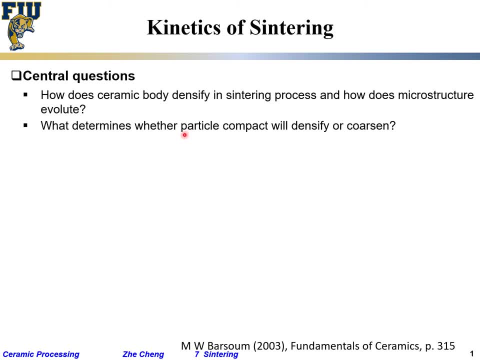 what determines the particle compact, Whether they would densify or whether they would grow only in particle size. cotton okay, And people have tried, but this is complicated When you deal with practical systems. there are many, many factors that are not very well. 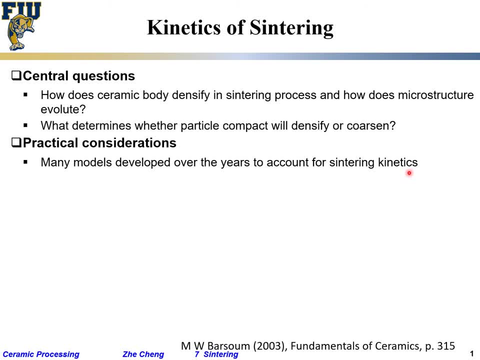 controlled come into play. Over the years people have developed many more models to try to explain account for the observed centering behavior, But there are many complexity or complications due to in real system. we have many other factors that are not very well controlled or even well understood. 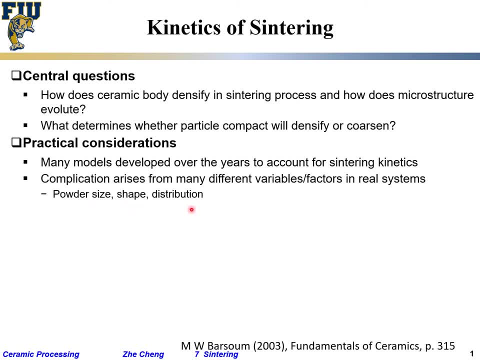 Powder size, powder shape. powder size distribution. Can you exactly control everything? to be spherical? Only under very rare cases? Typical is messy, Close, but not exact right. Can you control the size exactly? One micron, one micron, one micron Boy, not really right. Size distribution related. 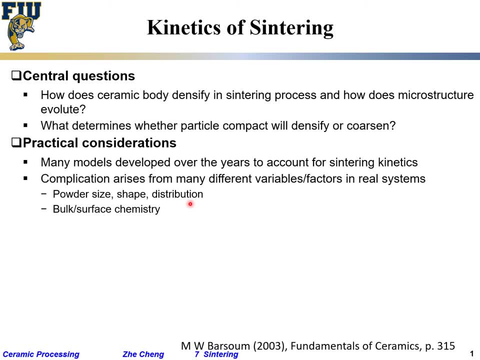 So that makes your model very. whatever model you build, you assume certain geometry, certain size, but in reality it's a mess. Okay, And about kind of surface chemistry, do people understand all the surface energy, all the surface diffusion property? No, Wait, Quite often the numbers are, if you are lucky. 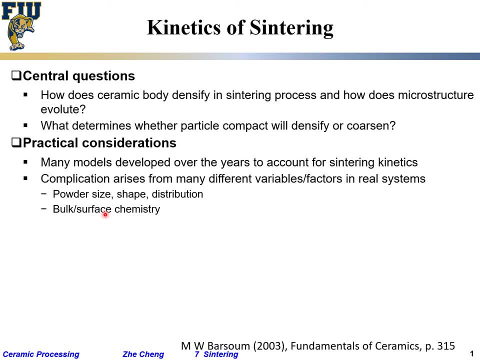 you find some number. Most cases you can find for new material or less common material. you don't have any number about them. Okay, In terms of surface energy, in terms of the lattice diffusion coefficient, not to mention surface diffusion coefficient, You have no idea what those are. 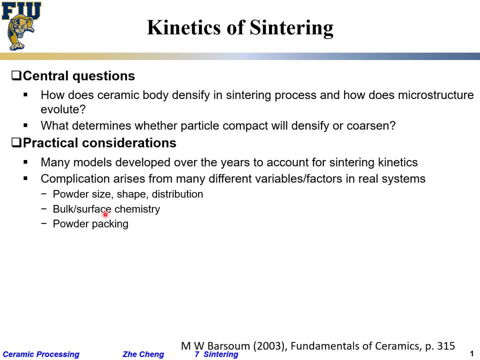 Powder packing, random packing, ordered packing. Ideally you can deal with ordered packing very easily, Random packing: okay, you have to build into the randomness, but that as complexity, Okay Additives, Quite often people addischeasés. nty-ade. add whatever other things into it That complicate, complicate- Right Initially, you, you don't know the chemistry for your other things into it that's complicated, right Initially, you, you don't know the chemistry for your. 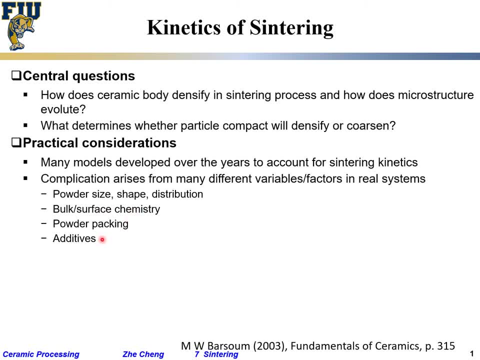 bulk of your material and then adding something more to it makes it even more complex. and the heating cooling schedule. well, we talked about isothermal sintering, but then the next thing we tell you is it's not exactly isothermal, because it takes time to heat up, takes time to cool down. 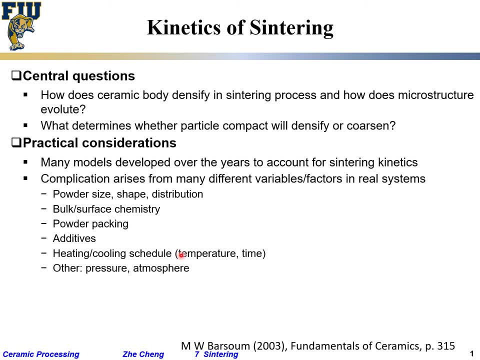 right, nothing is exactly isothermal and the pressure atmosphere, those things are also very tricky to control, very tricky to control. we are talking about atmosphere. okay, outside certain atmosphere, but within the bulk. if your ceramic body has certain size, within the bulk, the 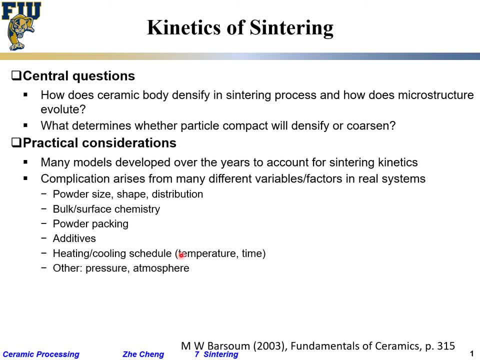 atmosphere clearly would be somewhat different from outside. and pressure? let's say you are doing hot pressing. can you guarantee the same pressure throughout the material? not at all. due to friction, due to the body and the size right. all these complications make the models. 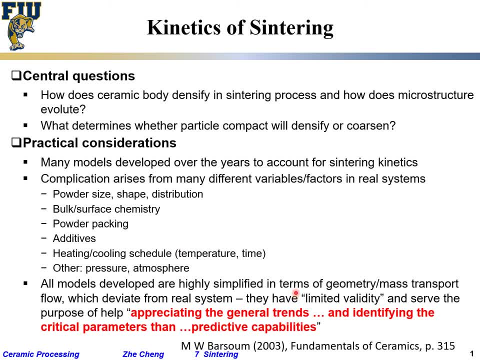 limited. they offer only limited guidance. you cannot predict very well. so for practical systems, the models, despite all the effort in developing them, they offer limited validity. you don't over generalize. I have this model. I can predict not exactly it's more about. 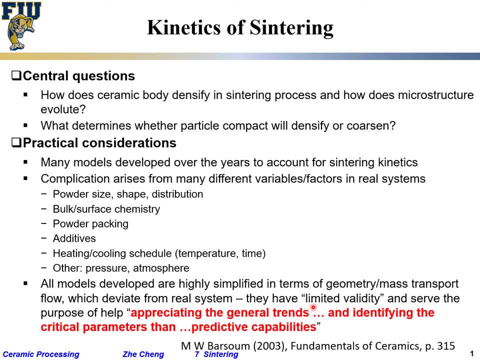 help you to understand the trend. of course, the higher the temperature generally, the faster the century, something like that that gives you a feeling. but well, temperature 1650 versus 1680, no, you don't know that level of precision. okay, identify the critical parameter. 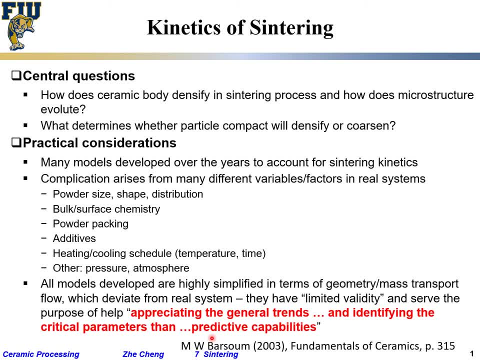 you know, okay, temperature is important. you know time is important, you know atmosphere is important, you know pressure is important. but can you exactly predict? I plug the number in the model will tell me what's my resulting: temperature, relative density. no, it will never be that accurate. okay, so it doesn't exactly have. 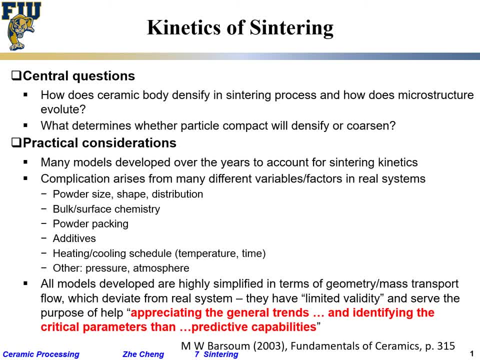 the predictive capability, but just help you. okay, these are the knobs, these are the trends. I don't go to extreme. right, that's the. you have a trend, but quite often, beyond certain points, the trend burns. we mentioned the centering. you can, centering not, you do, centering not at too. 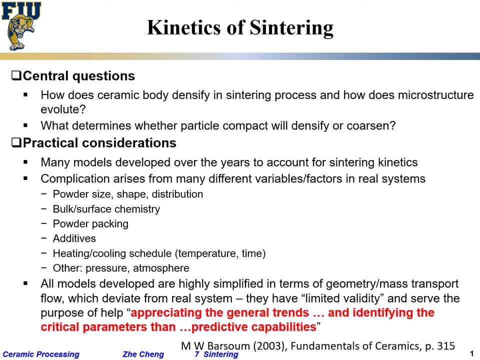 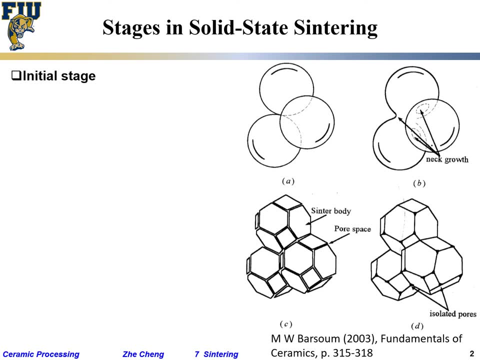 low temperature because you never achieve full density, but at the same time you don't also do it at too high temperature, because for those quite often you cause them too quickly and towards the end you do not achieve full density. okay, and people also try to build a geometric 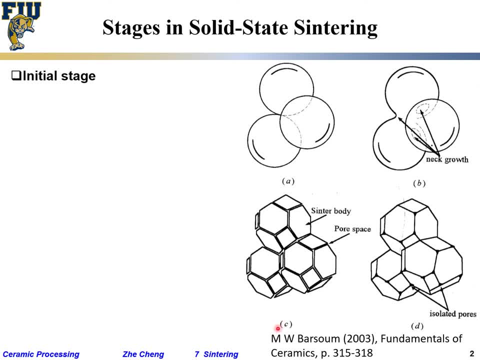 models to understand it. so when I borrowed some schematic, initially, ideally assume they are sphere touching each other only at a point. right, you are talking about real spheres that are touching each other only at one geometric point, which is mathematically even non-existing, no area, and then, after a certain time, of course, 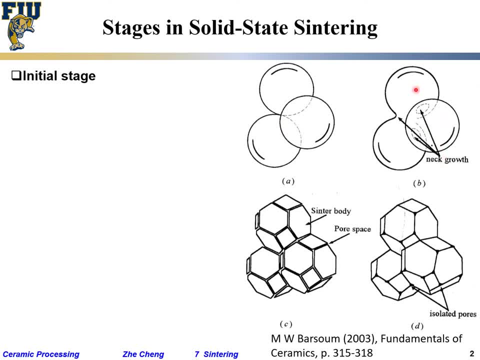 we would develop so-called neck between the point. now it enlarges into a finite area, we call it a neck. okay, that's initial stage in the particle contact area increase from essentially zero to roughly 0.2.. 0.2 versus okay over, maybe, the projection area. when you say 0.2, what does that point? 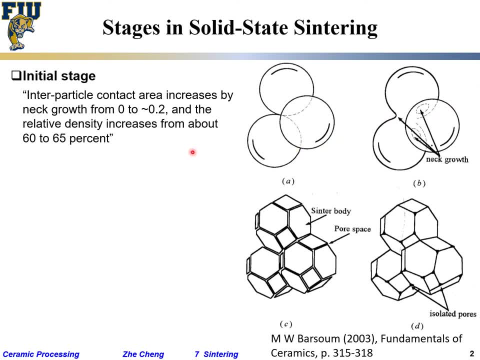 I'm probably projected area between those two. okay, and in that case the density doesn't increase too much. initially sphere packing- depending on what type of packing- you're roughly 60,, 55, all the way to 65, something like that. but let's say you're 60, and after a little bit of neck, 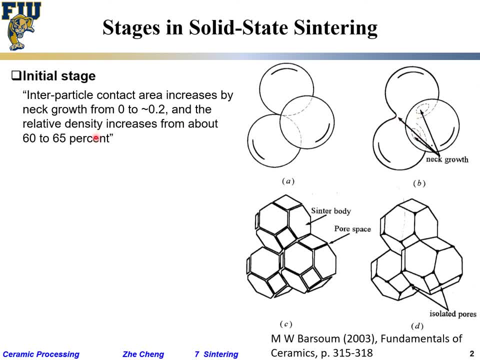 you go to 65, something like that, and then intermediate stage sintering. now the particles can no longer because they touch each other flat, it's no longer a sphere and people change the shape, started to do like a cube. 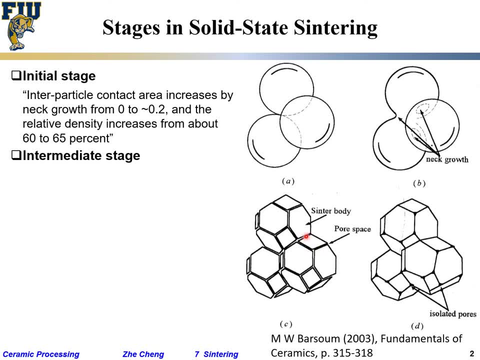 you start to cut corners, flat corners of center body, but then between center body there is a connected network of you. imagine the pores like a channel. okay, continuous pore channel. these things connected all of them together. when the relative density is roughly 65,, all the way to 85,, 90 percent. 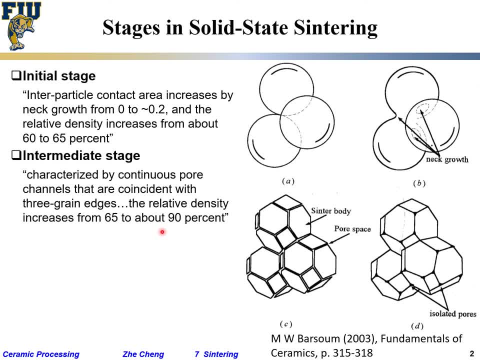 highly conceptual. okay, roughly, and during this time there's not much change in grain size. density would increase. but remember what we said: in the ideal condition the grain doesn't increase too much, okay. And then towards the end, towards the end, the connected pores now become isolated. 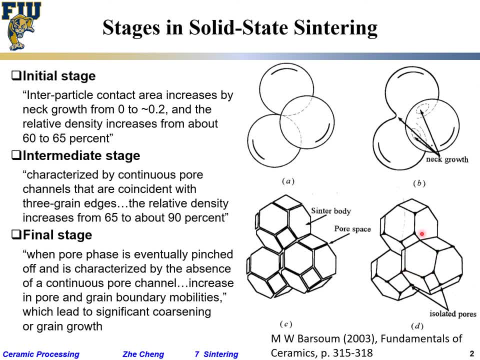 and only at the corners that they touch each other. okay, Connected They become from connected to isolated pores At the same time. this is not accurate. very good drawing. the particles should also become larger due to the unavoidable green growth towards the end. okay, So this is kind of. 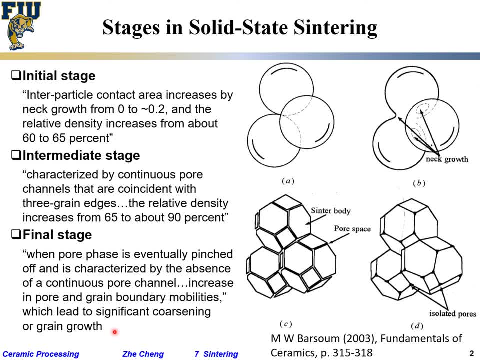 like how you imagine the process, but only for descriptive, nothing predictive. okay, But roughly from here to 80, 90 percent the grains hopefully don't increase too much, but towards the end the grains would increase. Over here the pores are still more like. 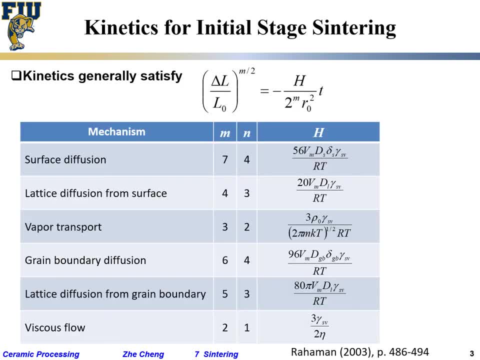 less connected, okay, And then people develop more sophisticated mathematical model. We don't go into detail, but you can see, depending on the different so-called mass transport mechanisms, people would have different non-parameters for the H-factor as well as for M and N. I made a mistake here. I have to check which one is M and which one is N.